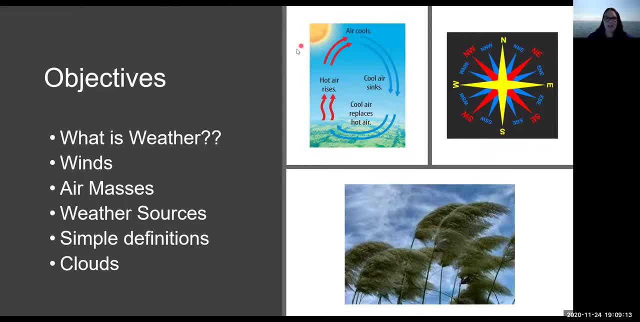 and then, depending on which way the wind is blowing, what are we likely to get as far as weather is concerned? A little bit about weather sources. I'm also going to show you some of the weather sources that we're going to talk about, So we're going to have a look at. 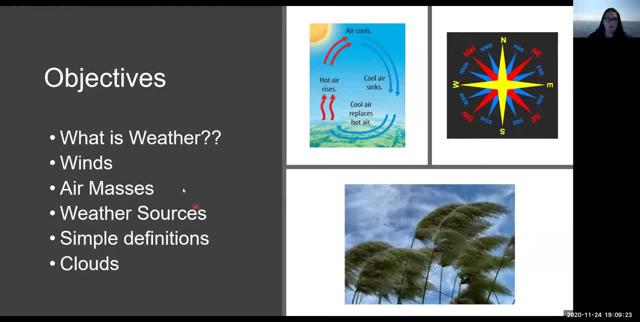 some of the weather sources that we're going to talk about. So we're going to have a look at different online sources, hopefully, and get some online sources working to give you an idea of where you could go get your weather from. I'll pause it a little bit later as well. be interested. 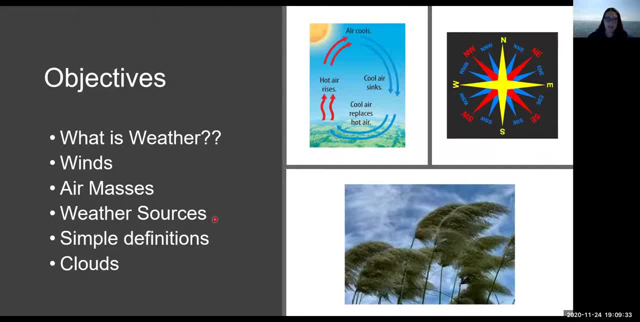 to see. perhaps I'm sure you guys have got some great online sources as well. We'll talk a little bit about some simple definitions and once we've done the simple definitions, I'll get you into some cloud spotting, and it will just be a bit of an introduction really into cloud spotting. There's 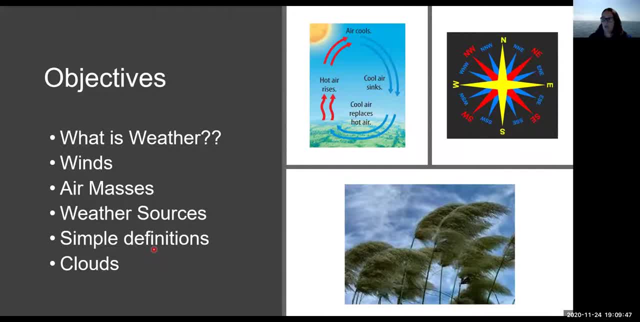 heaps and heaps of stuff to do with with clouds, but we'll just do a quick introduction. So for those of you who are new or are new to cloud spotting, I'm going to show you a little bit welcome. This is one of our bite-sized sessions, done during lockdown too. I'm Kath Scott. I'm the. 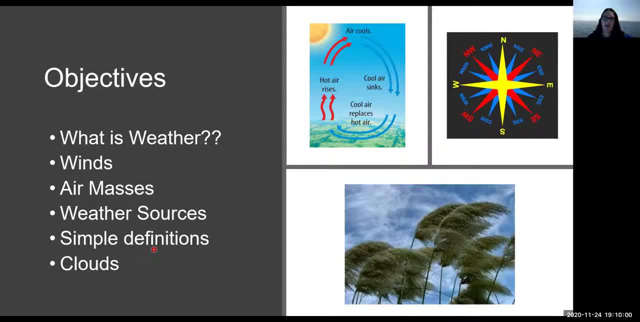 chief instructor here for Comfort Sea School and we're based in Portishead, just outside of Bristol in the southwest of the UK. I'm an advanced power boot instructor. I'm also a yacht master instructor of power and a shore based instructor, and one of my absolute passions is to teach weather and to 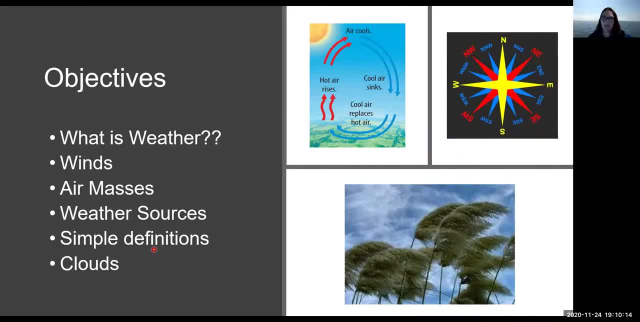 get people understanding weather, because, although it seems, on the face of it, quite complicated, there's just little pieces that you can learn that can make your sailing, your boating activities, a whole lot safer and a whole lot more enjoyable, most importantly. Okay, so that's what we're going. 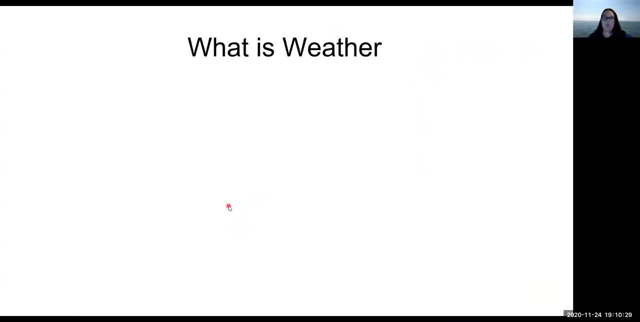 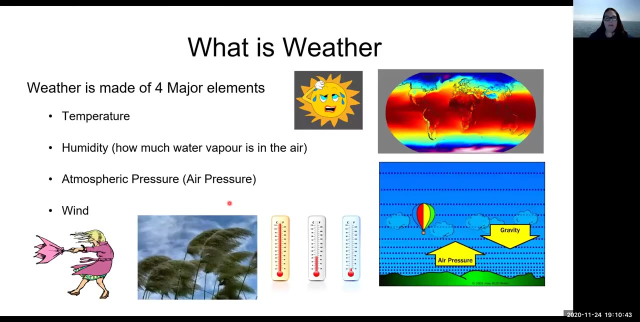 to take a look at this evening. So first of all, we need to say what is weather and just give you a minute or so to think. what do you? what do you think the weather is made up of? Where do we get our weather from? What constitutes our weather? So we've got the four major elements and this is 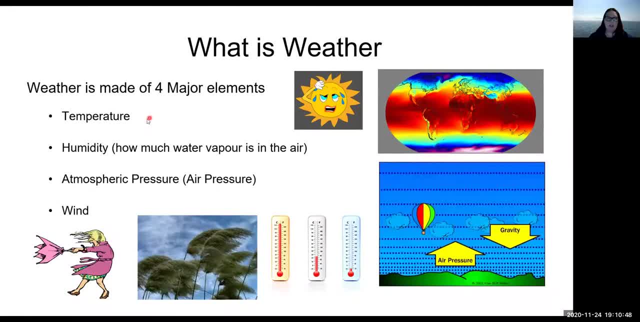 what creates all of our weather. We need to create. we need to have some temperature, and not just temperature, but some temperature differentials. You've got the chart on the right hand side of the the slide here showing you the differences between the very hot temperatures around the equator going. 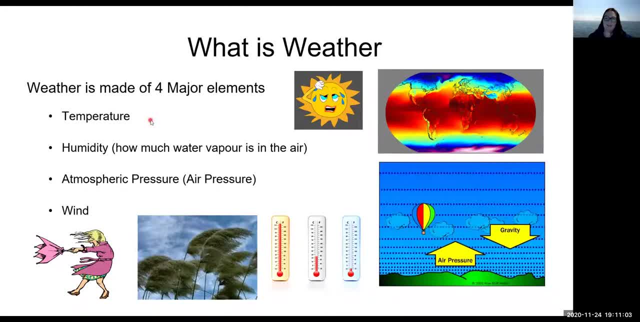 to the colder temperatures at the poles, and our temperature differences are also going to create some of our weather. We have our humidity, then how much water vapour is in the air, so that's where we can get our misery rain, that's where we can get lots of rain, and we also have our 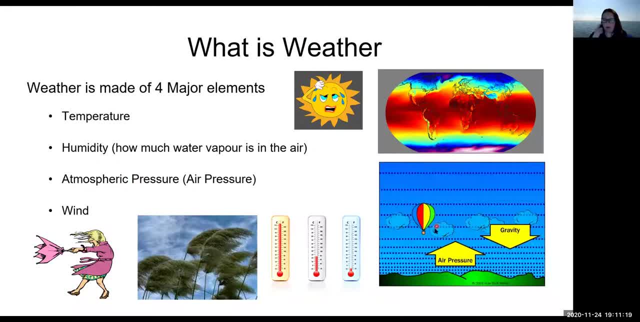 atmospheric pressure. so our air pressure. We'll talk a little bit more about our air pressure a little bit later, but effectively we've got our air pressure and we've got our gravity. okay, and that's what's going to get our hot air balloon flying- and more of him- a little bit later. 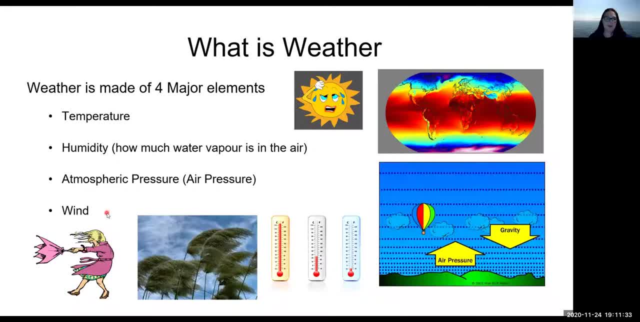 And we also have our wind. so if we combine the temperature, the humidity, our air pressure and the wind, that is really what creates our weather and in different levels, will give us different weather. So something that has fairly low humidity, with some nice high air pressure, with some very 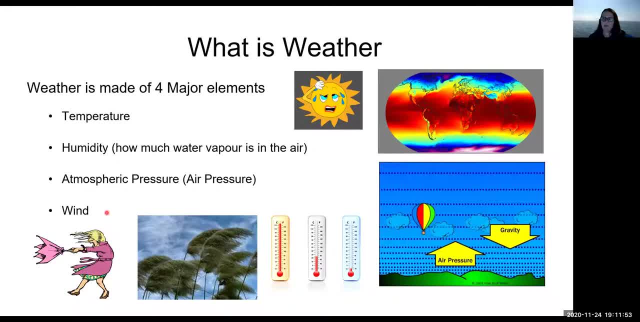 good wind and some nice temperature would be great barbecuing weather and probably some great motorboating weather. however, not so good if there's no wind, if I want to go sailing. So from that perspective, we have the four major elements and the different elements that we have, or the 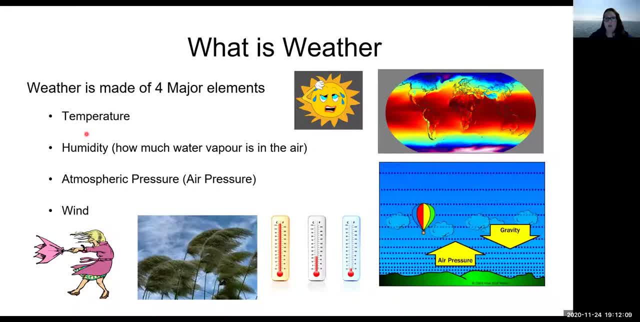 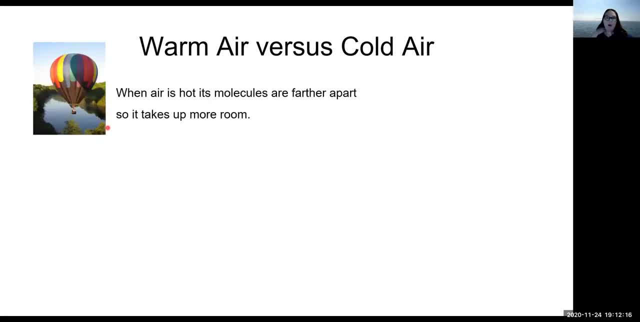 amount of the elements we have is what's going to create our weather. So what does it mean as far as our warm air versus cold air? So we'll start with our hot air balloon. How do we get our hot air balloon to rise? 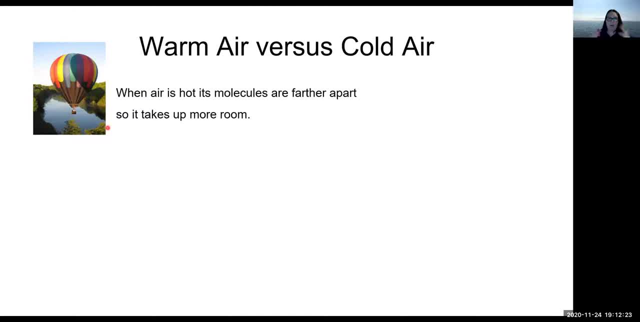 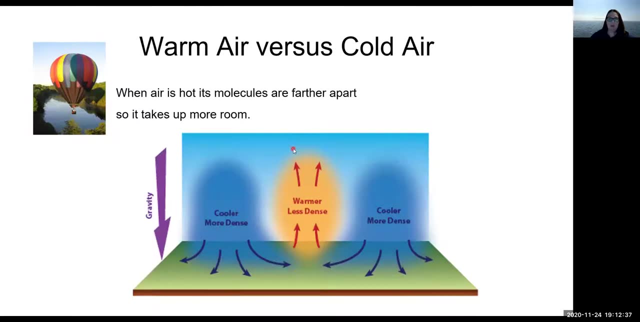 So we have to get more hot air into it. The hotter the air, the further apart the molecules go, the larger the balloon becomes, It takes up more room and the balloon starts to rise. The hot air is lighter, it's warmer, it's less dense and therefore it starts to rise. But if we take our 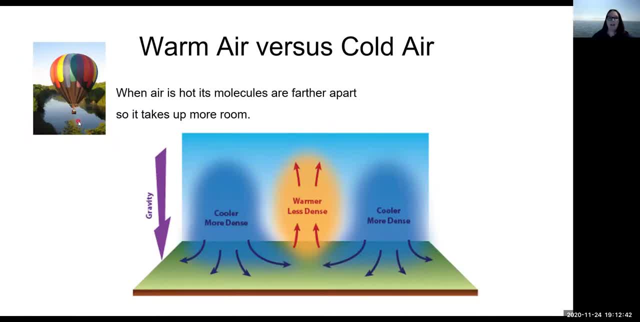 hot air balloon analogy. we have to keep firing the air into it because the air starts to seep out. So we need to keep it warm, we need to keep it nice and dense and we need to keep it with the molecules further apart. That's how our hot air is going to rise. 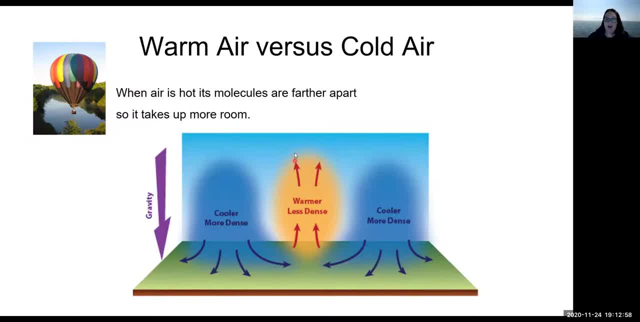 So, equally, as we have our hot air rising, the further away from the land it goes, the more it's going to cool up in the atmosphere and we're going to have cooler, more dense air And, effectively, what we're looking at here is high pressure and low pressure. 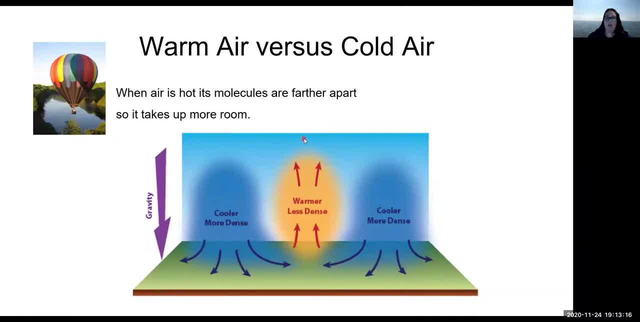 So we're looking at the air being sucked up because it's starting to rise and, as it's starting to suck up, we're creating a vacuum here which is going to be filled by cooler and more dense air. okay, so think hot air balloons, think um bonfires, where you see all the hot air rising. okay, the hot air is. 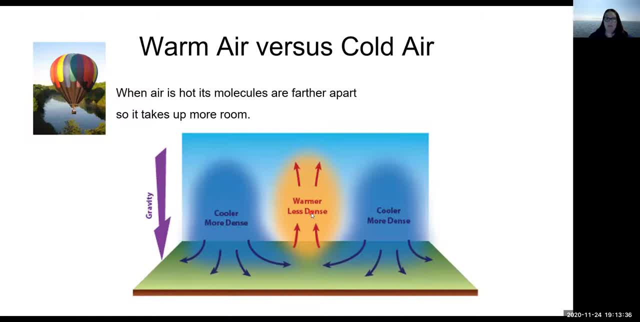 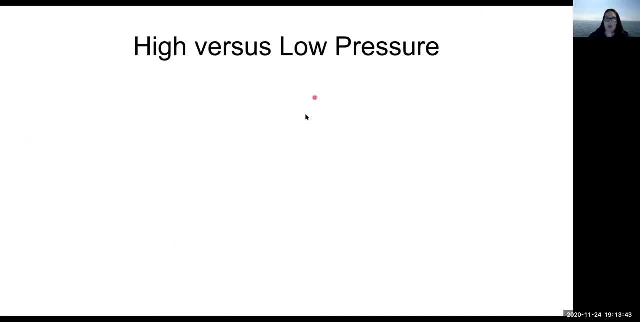 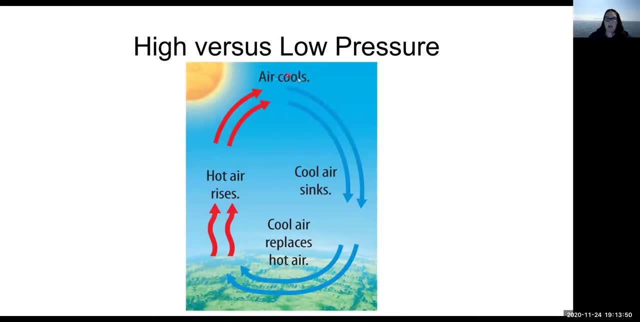 going to rise and be much less dense, take up far more space than our cold air is going to. so how does that get into our high pressure versus low pressure? and this is a really simple picture. here we have our hot air rising. as it gets higher up into the atmosphere, it starts to cool and the 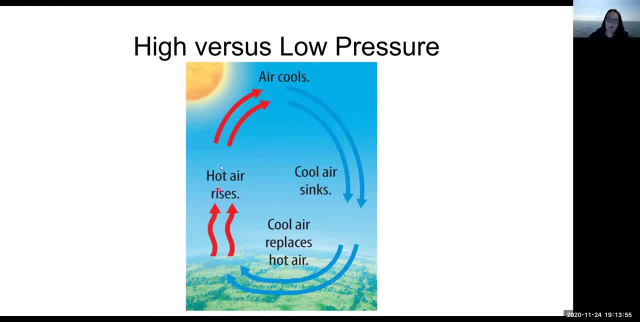 cool air sinks, and the cooler then replaces the hotter. so we sort of get this cycle that goes around, and the more the hot air rises, the more it cools, the more it starts to sink. and if we think of it in simple terms, then as it rises it's not pressing down as much onto the the earth. okay. 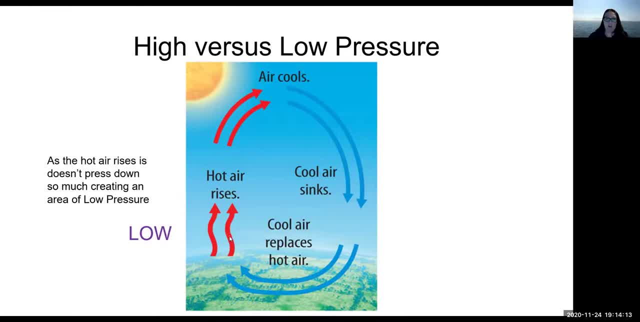 so it's creating in here an area of low pressure and as it starts to cool and it starts to sink on this far side, then we've got the cold air sinking down into the atmosphere and the weight of the air pushing back down onto the earth's surface and creating an area. 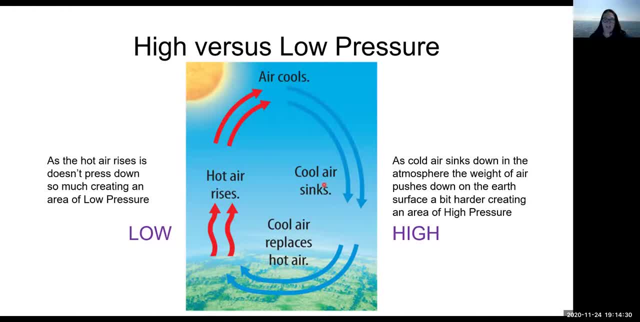 of high pressure, okay, and what we tend to have is our wind blowing from high to low pressure, okay. so the wind is blowing from high to low pressure in this place. it's replacing that hot air as it rises, because it's created a bit of a vacuum. 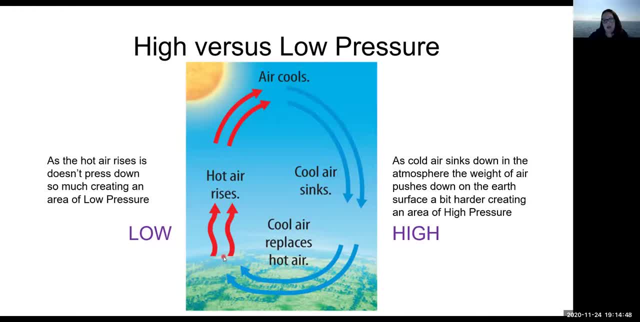 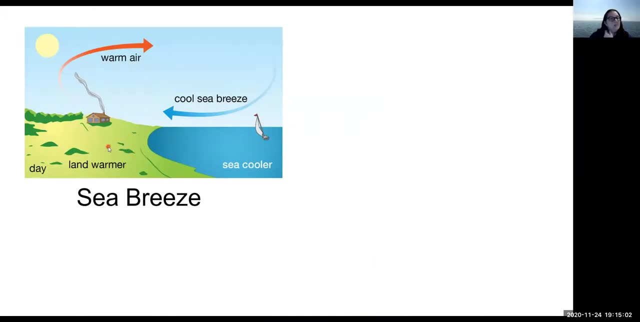 so if we can understand low pressure, high pressure and the whole air cycle, what we can understand is why we get sea breezes and land breezes, okay. so this is where we start adding a little bit of the wind in. so here is our typical sea breeze, our typical sea breeze by day we've got the sun beating down on. 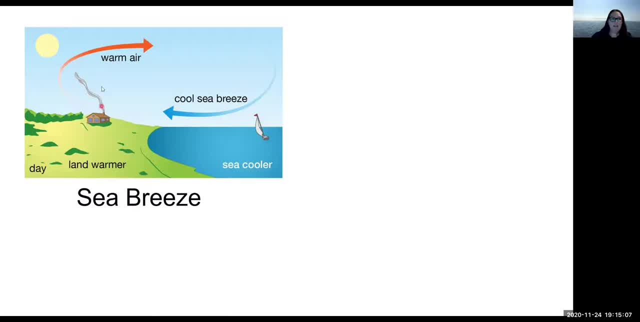 the land. it's heating up the land. it's creating warmer air. the warmer air is rising and as the warmer air is rising, it's going to be replaced then by the hot air. so we've got the hot air, the cooler sea breeze, because the sea isn't going to heat as quickly as the land will be. 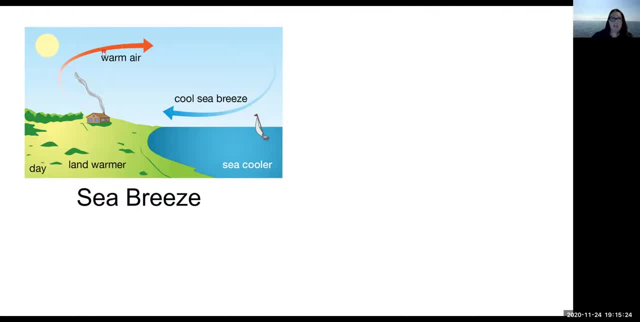 and as the warmer air rises, it's also going to start expanding. it's going to start expanding out and as it expands, it's going to start to cool the higher it gets and it's going to start to create this cycle. okay, but how does that relate to our high pressure and our low pressure well as 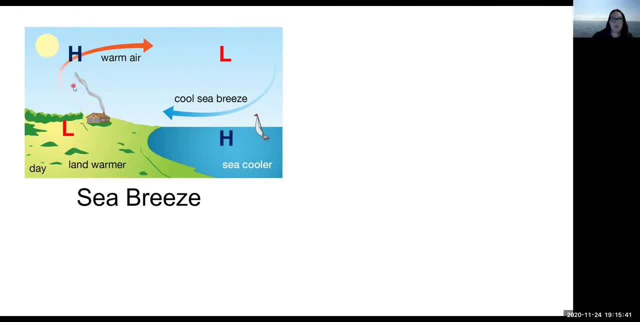 the air starts to rise. it's creating low pressure, which is creating that absence. then it starts to become so. it's unstable. it starts to cool down and it's going to start to cool down and it's going to become a little bit more stable. then we have our low pressure and it calms down into our high. 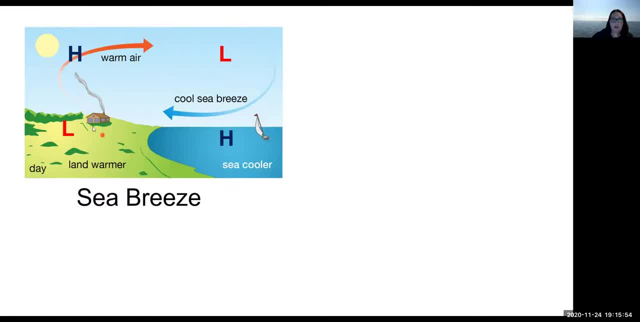 pressure. so we have that whole cyclonic, if you like, that whole cycle that's going on here. so we know that if we wait until the afternoon, the hyper there, the sun, will have beaten down onto the land, it will have heated the land more than the sea and because of that it will have started to create. 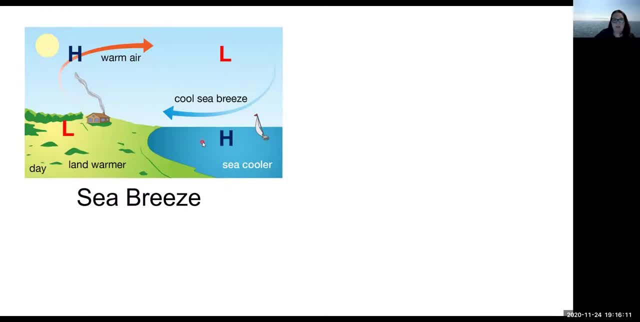 this cycle. okay, the bigger the temperature differential then between the warm and the cool, the stronger the breeze will be. so if we've got a much, much hotter hub air rising here and a much cooler sea, so around to the spring time perhaps, when we're starting to heat the land and the sea is a little bit cooler, we're going to 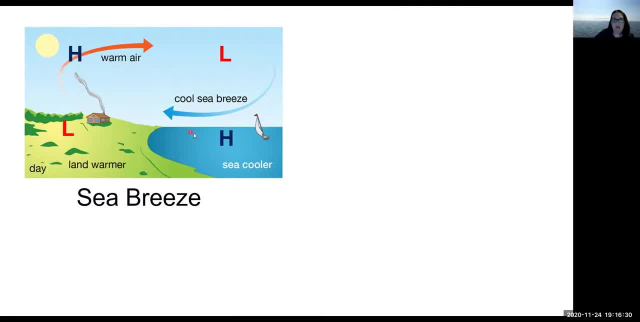 get a much stronger breeze coming in on our sea breeze. how does that work? when we're looking at our land breeze then? so this is our night time. this is where the sea is going to retain its warmth and the land is going to cool. and if you look now, we've got a slightly different cycle where the 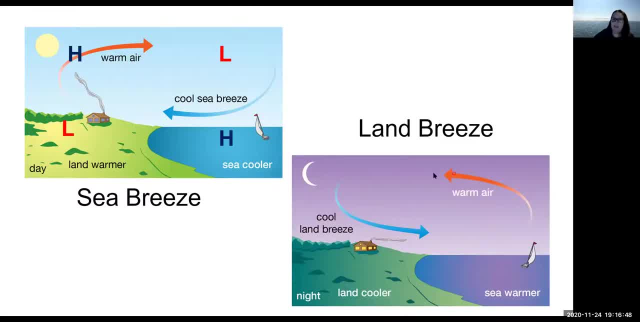 warm air is still rising and the cold air is still rising. and the cold air is still rising and the wind is still blowing over the over the sea story. it's creating an absence and it's going to be filled by that cooler land breeze as the land cools down. okay, and again we've got our low. 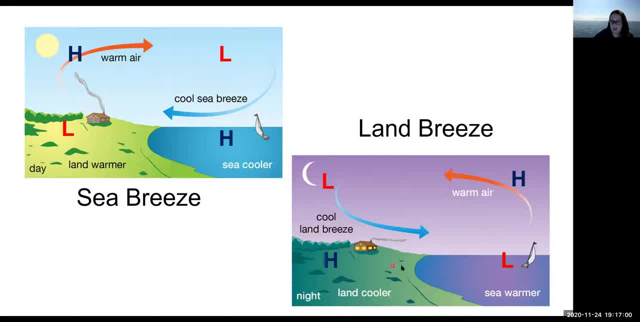 pressure as the the hot air rises and our high pressure as the cold, cooler air sinks down. so that's the fundamentals of our wind, if you like, and our wind, our breeze, is created, blowing from high pressure to low pressure, but as well as that, we have our some global winds. so the fact that the earth is rotating is giving us that coriolis. 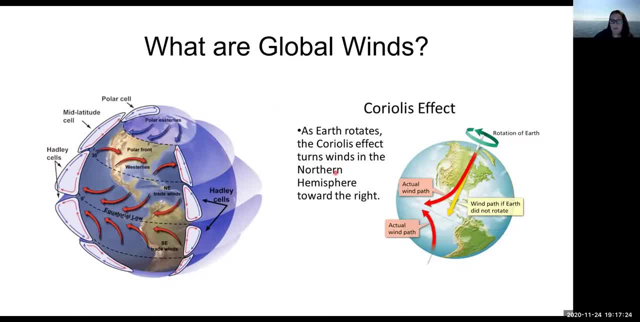 effect. so we're having winds in the northern hemisphere genuinely turning towards the right, and that's what creates in our cells. this is where we have our warm rising and our cool sinking, and this is all to do with how it's heated by the sun at the equator. we've got these different types of 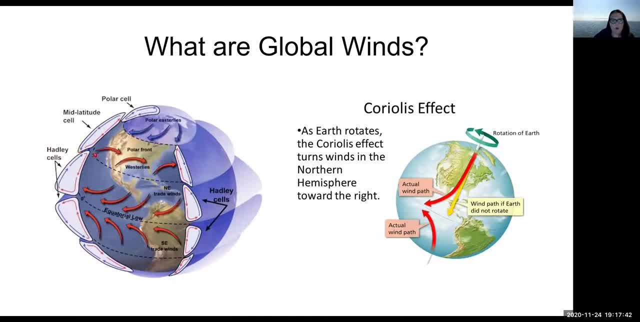 cells and within those cells, and including our coriolis effect. what we end up with is our trade winds, showing you predominantly the wind that's going to be blowing from high pressure to low pressure in each of these different latitudes. okay, so if we're looking at the trade winds here, 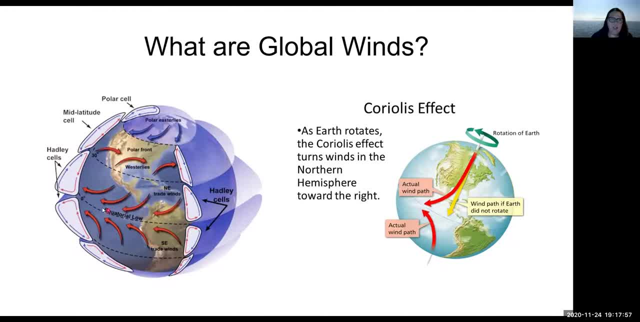 or just above the equator, or above the equator, sorry. we've got the equatorial low where we're creating that low pressure as it rises. we've got northeasterly trade winds, given how the world spins, and at the moment I think it was either yesterday or the day before the arc set off. 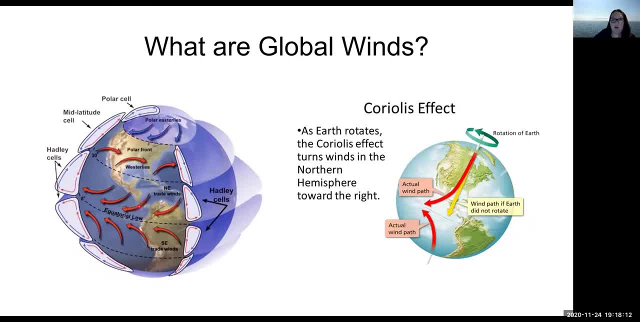 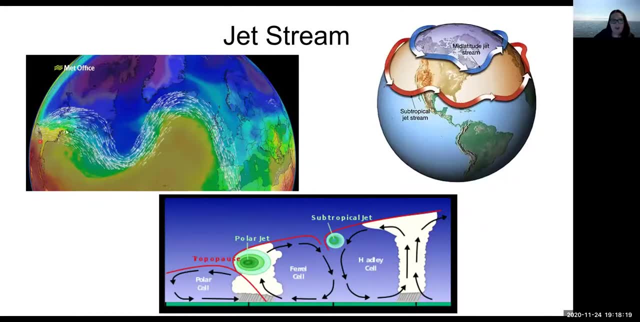 and the arc are going to be sealing those trade winds across towards the caribbean. okay, so we've also got our jet stream to look at then. so here is our jet stream, and this is really a big supercharged conveyor belt of higher level air could be up to about 200 miles an hour. we've got. 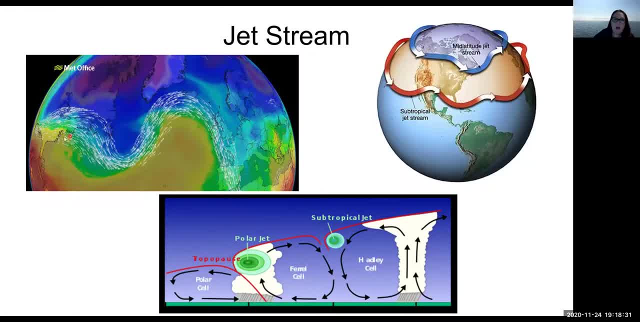 two, we've got the mid-latitude jet and we've also got the subtropical jet, and what it does is it drives our pressure systems. so i actually think of this a bit like a conveyor belt. this is what's going to bring our weather systems. we've got a little kink in it here. just coming over to the 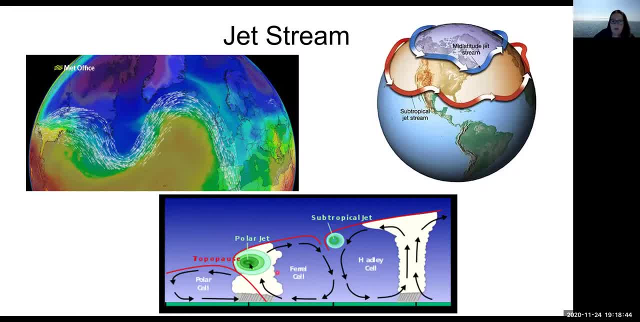 top of the uk and this is how it sits within our feral cell and within our hadley cell. we've got our subtropical jet here and our polar jet- okay, but this is really going to supercharge any of those systems, because it's effectively a 200 mile an hour conveyor belt bringing the systems across. 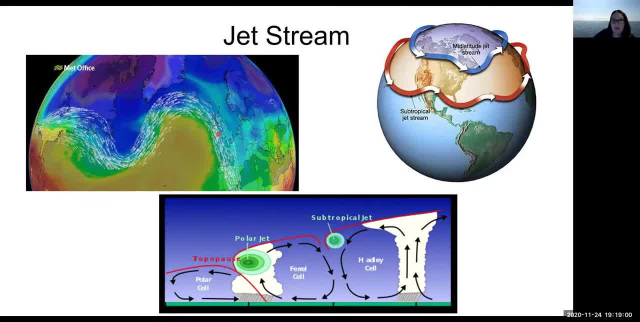 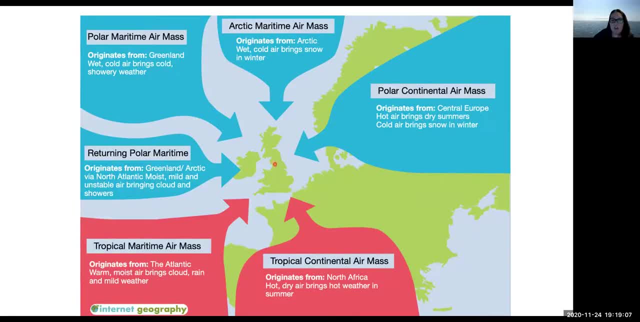 to us. so, as well as the warm and the cold, if you like, creating that wind, we've also got to consider our jet streams as well. but where does our air come from? okay, so this is looking at the uk, and what we have here is a whole different set of air. so if our air is coming up from the continent, we need to think if 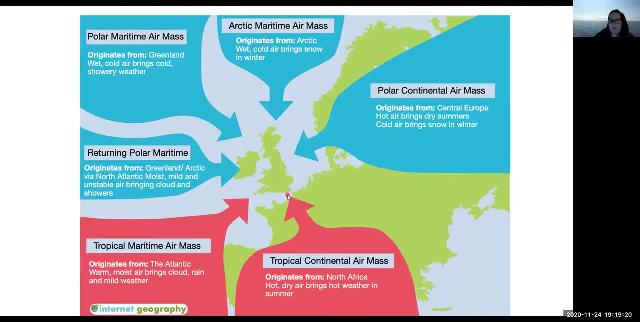 the air is blowing in over the continent. what would we expect? well, the air is coming over an air of a landmass. if it's coming from a landmass, it's not going to be particularly wet. okay, we need water, we need the sea to give us some fairly wet air. okay, coming up from north africa, it's. 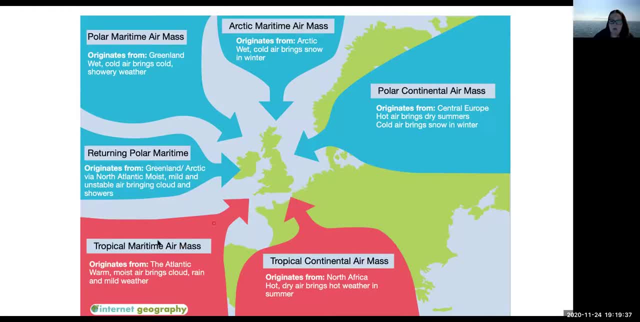 bringing in nice hot weather in the summer. okay, same with our tropical maritime air mass. this is still warm. it's warm and moist air, so it's going to bring in some slightly wetter air, if that's where our weather is coming from. moving further up, then, if we look at our polar, we've got returning polar maritime, which is where 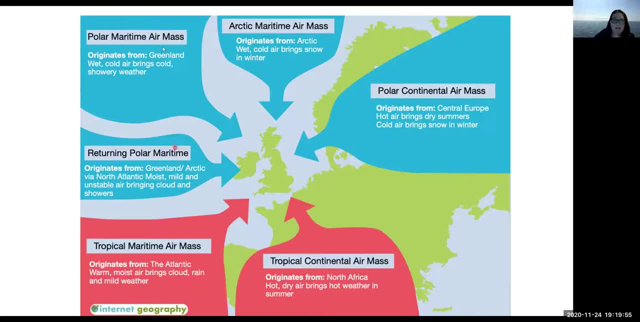 we have a cycle coming in around greenland and the arctic by the north atlantic. we also have our polar maritime air mass here coming in from greenland, bringing wet, cold air. it's coming across a big ocean. so if it's coming across a nice big ocean, it's bringing us wet, cold air. okay, our polar. 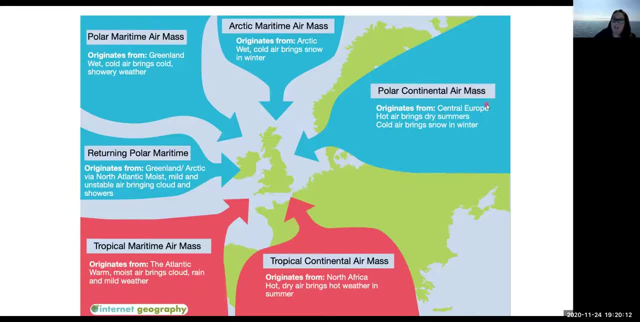 continental air mass. then coming in from north africa it's bringing in some slightly wet air. air from central europe is bringing us what would be lovely dry summers in the summer and lovely um snow in the winter, because the cold air comes in and it interacts with our warmer, moist air and 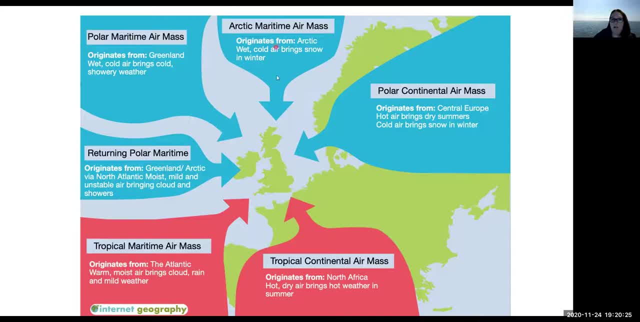 that's what's going to create a lot of our snow. okay, anything coming down there northerlies from the arctic is going to be cold. it's coming across um the ocean, if you like, so it's going to bring wet, cold air and it will bring us snow in the winter. so the direction that the wind is coming. 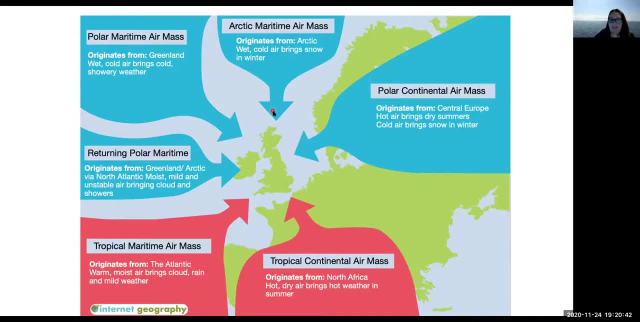 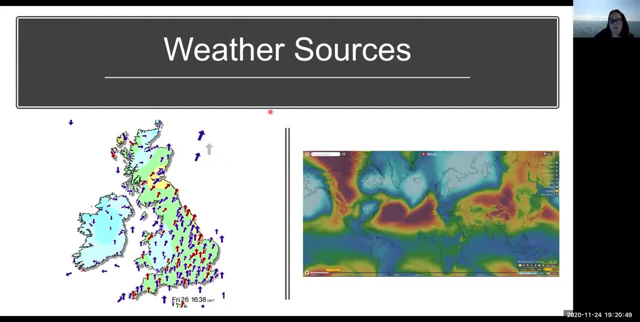 from and where that weather is coming from, is going to be a lot of snow, and it's going to bring a lot of heavy snow, and we'll give you an idea of what type of weather you could reasonably expect. so where do we get our weather from? well, there's heaps of weather sources. okay, i'm going to show. 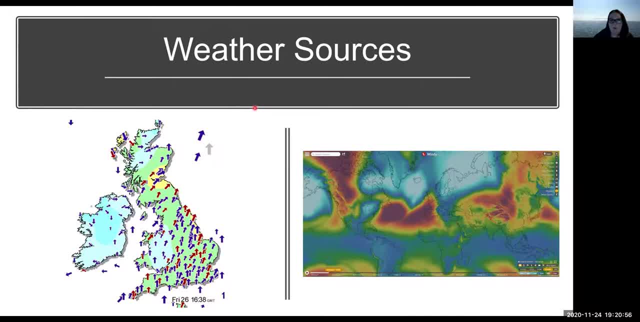 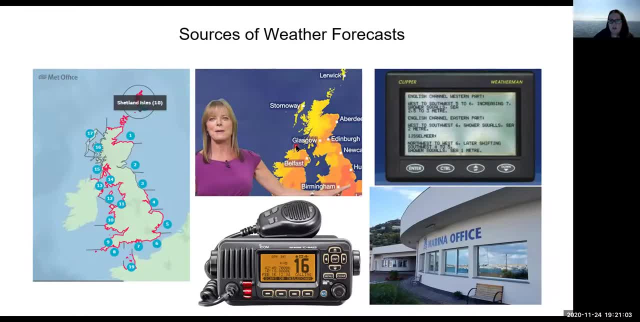 you just a few. i'm sure you'll all have plenty of weather, different weather apps, different weather sites and so on- but we're going to look at some real basic ones. we can get our weather from the television. so we can have a look at our weather on the television. we can get the the usual um after. 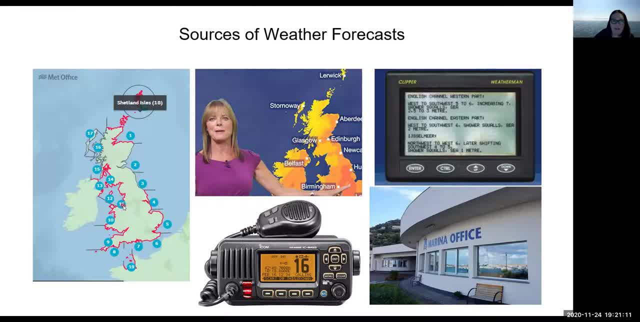 the news type forecast. we can get our weather from the television. so we can get our weather from the from the MET Office. we can have a look at something coming through, perhaps on Navtex. we can also get it from our marina offices. People often underestimate that going to the marina office. 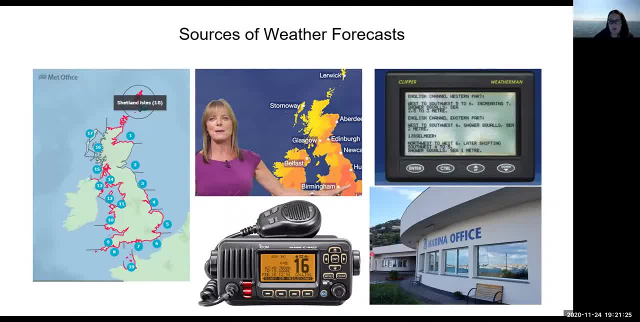 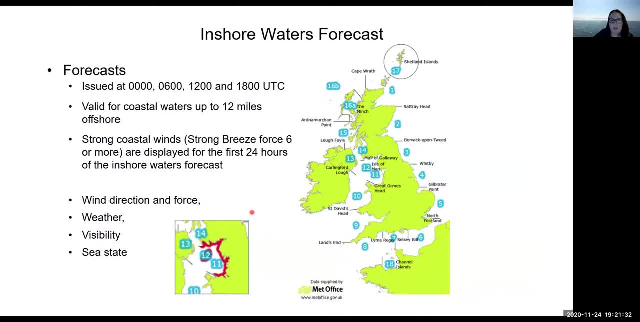 they will often have the weather forecast ready there for you, And we can also use our VHF radios in order to get the weather forecast. okay, And we're going to focus on just a couple. If we take a look at the inshore waters forecast, then the inshore waters forecast is all the 18. 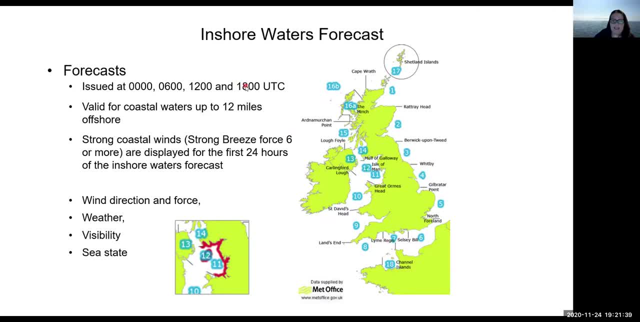 areas around the UK, issued four times a day, okay, and valid for coastal waters up to about 12 miles offshore. Once we get any strong coastal winds then. so we're looking at a strong breeze of 4.6. so both of 4.6 or more we're looking at displaying a red line around the outside of that particular. 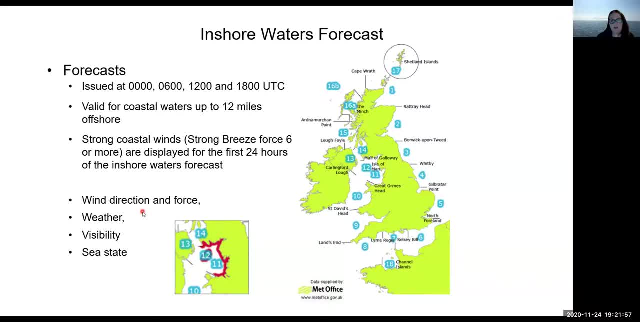 area, And what the inshore waters is going to give us is our wind direction and force. so what direction is the wind coming from and how strong is it blowing in both it And what the type of weather we can expect? So we're going to look at the inshore waters forecast and we're going to 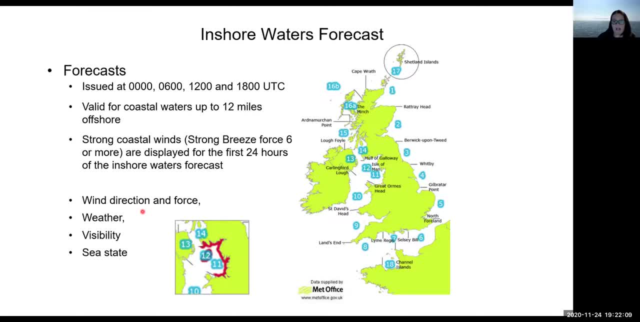 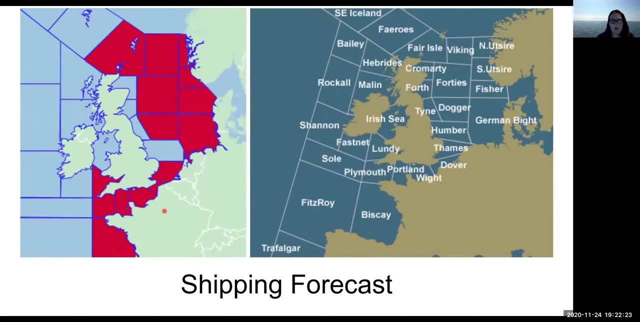 look at the type of sea state. so how is that wind going to interact with the water and how big or small will our sea state be? We can also look at something like the shipping forecast. and now we're going a little bit further offshore, okay, A little bit further offshore. so we're interested in the 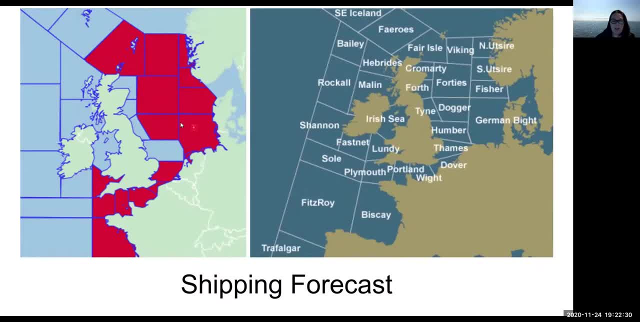 picture on the left-hand side here, Anything with a big red box, and it is looking at gale force winds, because previously we were looking at strong winds, now we're looking at gale force Winds again. any of these red areas showing that there would be a gale force wind predicted within. 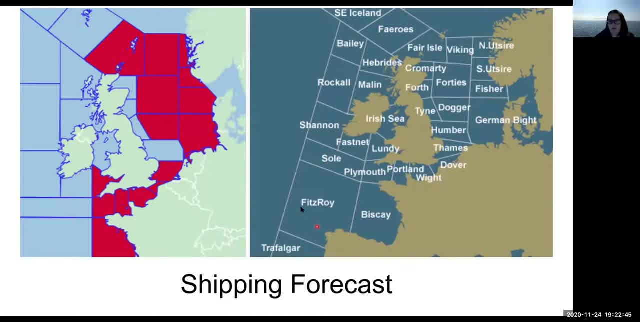 that particular period. okay, We've got all of the areas on the right-hand side here so we can listen to the shipping forecast to understand, perhaps, where our wind is coming from, where our weather is also coming from. So, coupled with our inshore waters, I'd also be taking a look at particularly 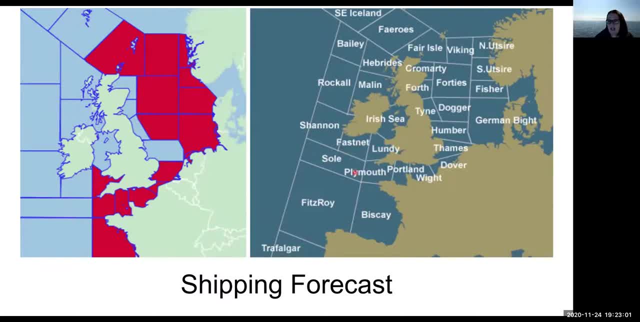 if I'm sailing down the Bristol Channel, I'd be interested in the areas of Fastnet, Lundy, Sol, Plymouth to find out where the wind is coming from. If I'm sailing down the Bristol Channel, I'd be interested in the areas of Fastnet, Lundy, Sol, Plymouth to find out where the wind is coming from. 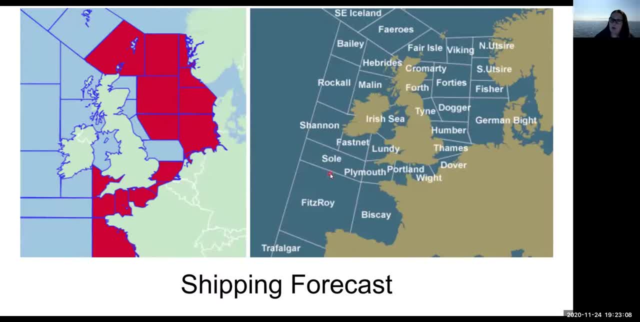 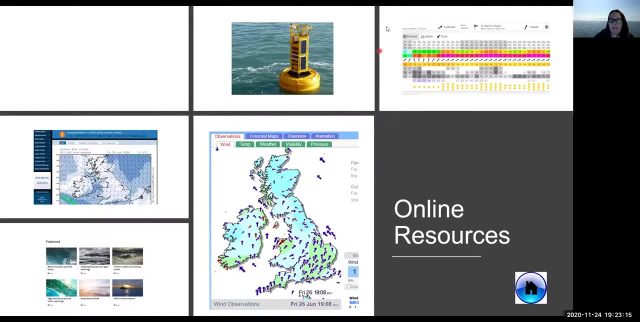 find out where there are, what our weather is going to be doing now, but also a little bit later, as the weather system is moving predominantly from the southwest. So we have a whole heap of online resources. if I just pause you there, what I'm hoping, just do, okay. so here we've got our 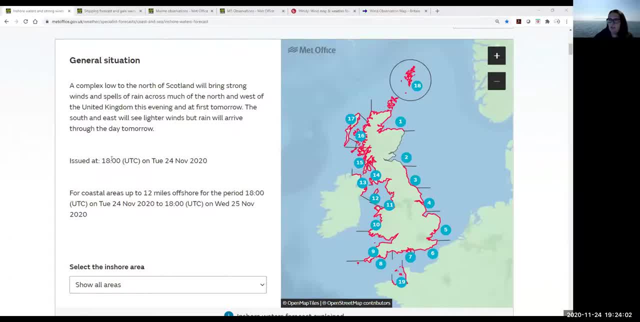 inshore waters forecast. this is the today's inshore waters forecast. you can see it was issued at around 1800 UTC. let me just grab my spot light. there we go. we've got our issued around 1800 UTC. we've got it for coastal areas up to 12 miles offshore, and also you can see that we've got quite a lot. 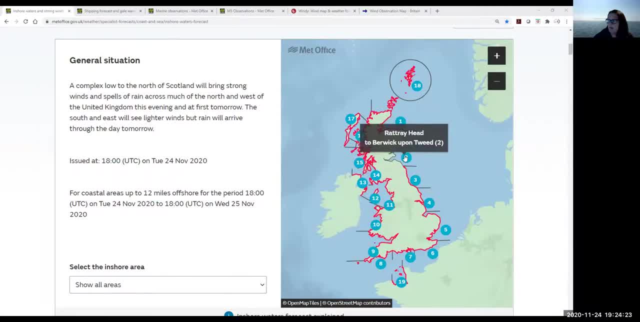 of red around the outside of the UK, apart from area two at the moment, which seems to be the only one without any strong winds on. okay, so if I want to select my local area and go to Lands End of St David's Head, including the Bristol Channel, and what I actually would want to do is I'm 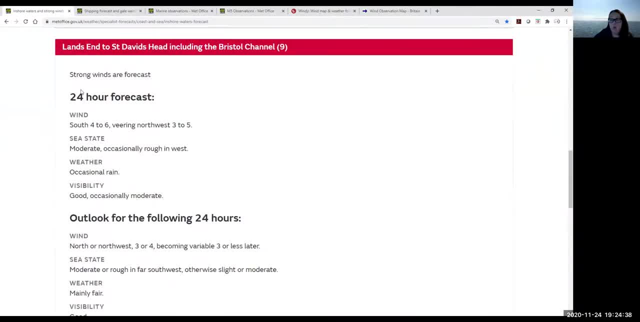 actually get, then is a little bit more information about it showing me what is actually happening already. there is a red bar at the top which is showing me that strong winds are forecast. I've got my 24-hour forecast. I've got southerly winds, four to six, veering northwest three to five. 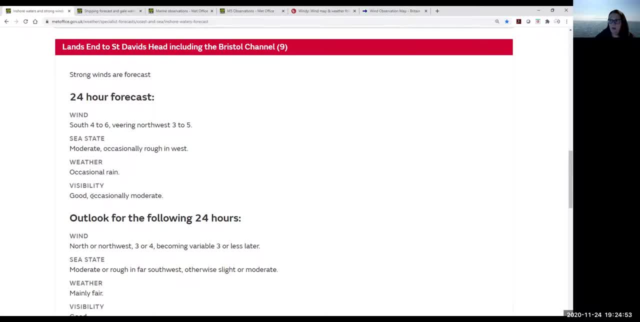 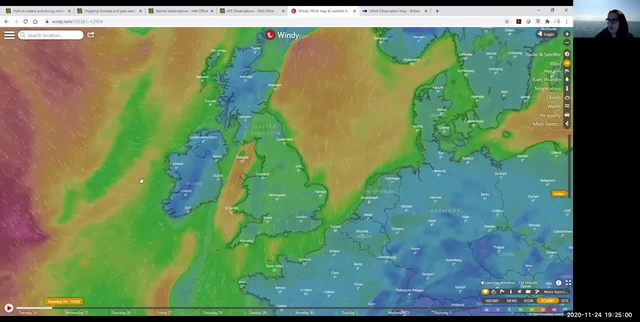 with a moderate, occasionally rough sea state in the west weather and my visibility, and also it's giving me the outlook for the following 24 hours. okay, if I change the screen, hopefully you can now see the windy screen. okay, this was a real revelation when I first found it. I think you. 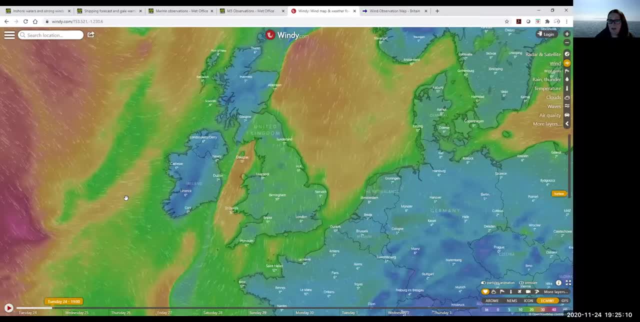 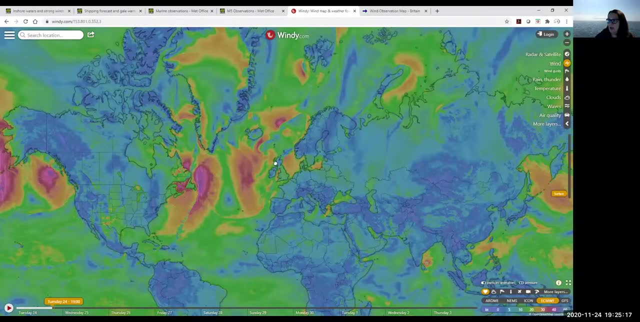 could probably lose many, many days of your life. if you look on on the windy screen it gives you a whole look at the weather in the world. we can zoom right out and we can go and get it pretty much the weather anywhere in the world. okay, I'll zoom a little bit back into the UK. 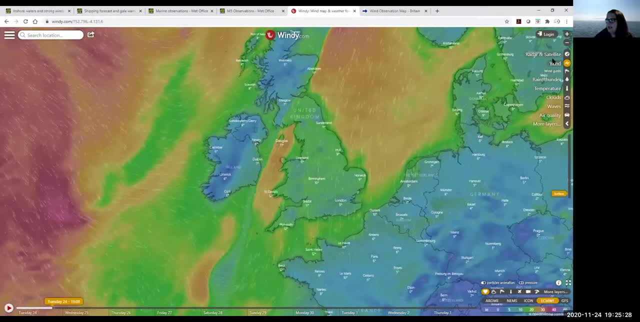 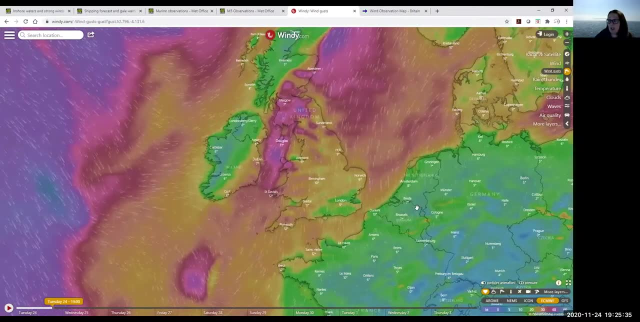 let's have a look, okay, and what I can do is on the right hand side. here I can change what I am looking at currently experience. I'm looking at wind. I could also look at wind gusts, so I can change that and the different color scheme down in the bottom right hand corner of the slide. there you can see the wind gusts. I. 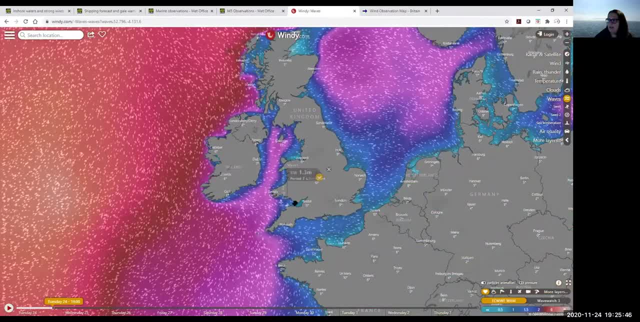 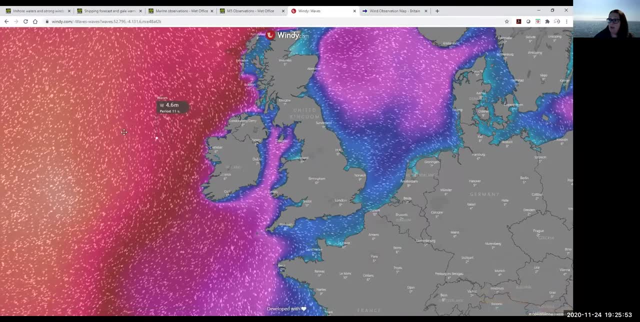 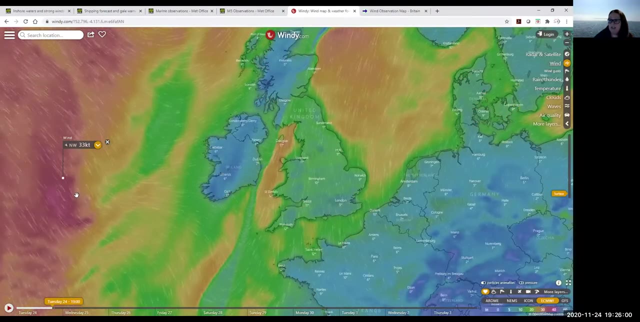 can take a look at the waves. I can also go and click on it and find out that currently, just off the coast here, we've got 1.3 meters for the wave height. out here it's going to be around about 7.6 meters, but that also tallies with the wind. we've got 33 knots of wind sitting out there, so we'd be 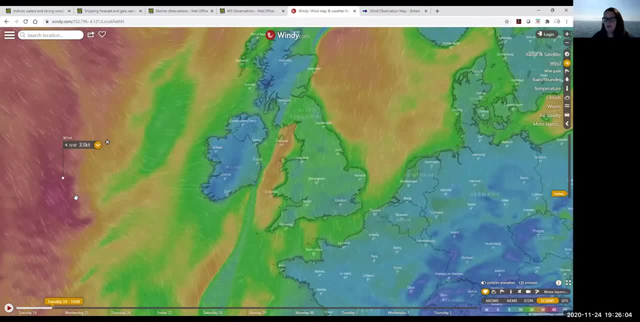 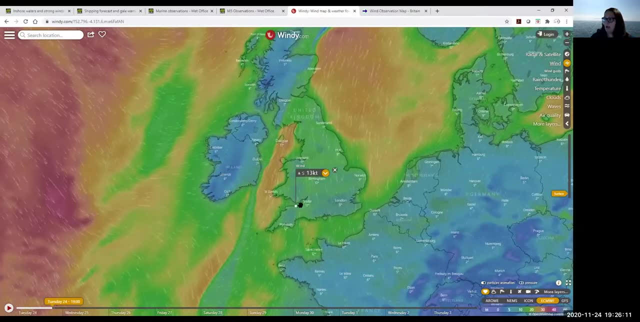 expecting that strong wind to be kicking up some fairly big waves, okay, and more about how that all works on the next session. but it gives you a good idea of where I can come in and I can get a nice little forecast. if I pop it further at the bottom of the screen I can get what looks like a whole 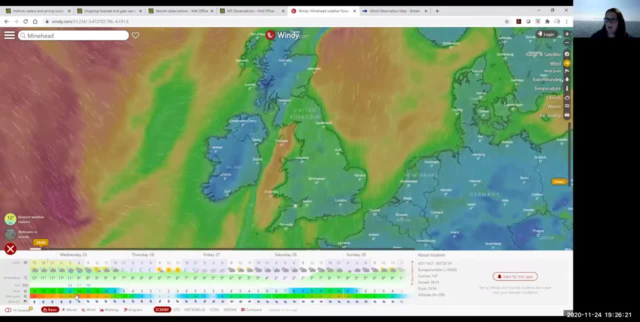 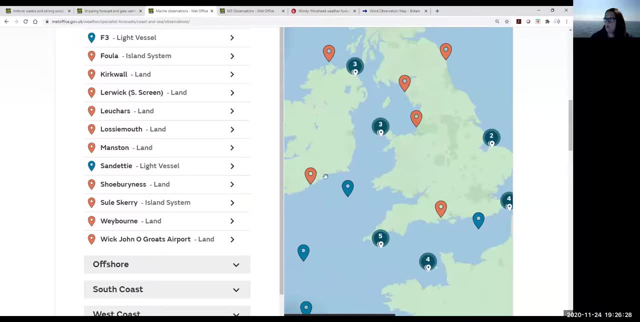 forecast out to Sunday. I can see what the wind speed is going to be, what the wind gusts are going to be, temperature, and so on. okay, I can also use something called the Met Office weather system, the weather stations. okay, and these are the weather stations that are going to be, the weather stations that are going to be the 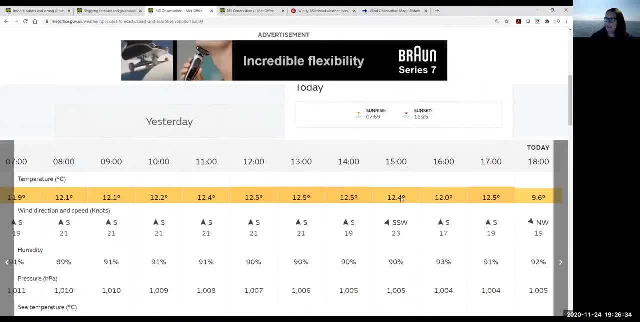 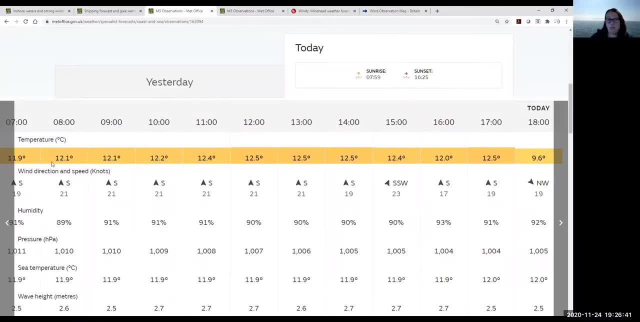 weather boys that are dotted around the UK so I can click on the weather boy here. this is the M5 M5 boy out in the Irish Sea, and what I can actually have is some up to the minute information which shows me what the what the weather has been recorded at that particular station. so all the 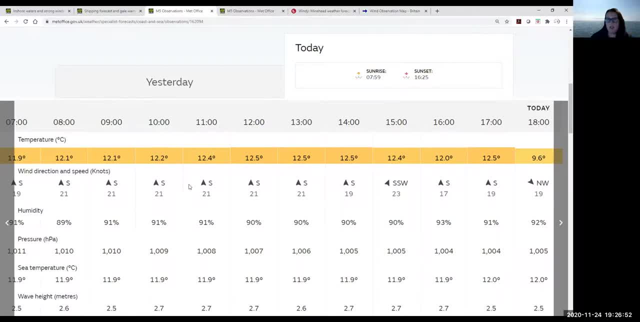 way up to six o'clock tonight. it gives me an idea of wind direction and speed. so, as well as those giving me a forecast, I can actually look at what is reality. so what is currently happening at that boy, and I can start to see what's going on. and I can actually look at what's going on and I can. 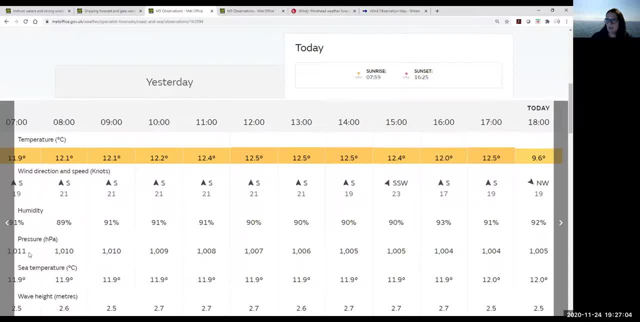 start to see what's going on, and I can start to see what's going on and I can start to see what's happening here. I can see the pressure at seven o'clock this morning was a packed 1000 and 11 and happening here. I can see the pressure at seven o'clock this morning was a packed 1011 and it has. 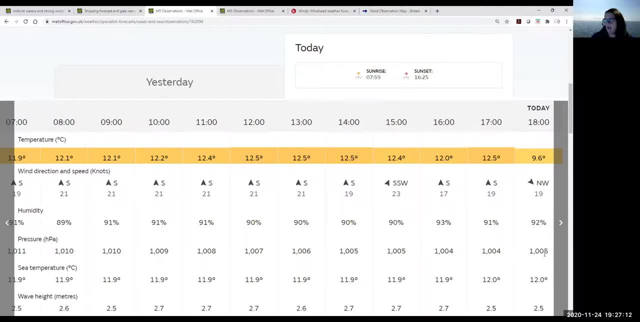 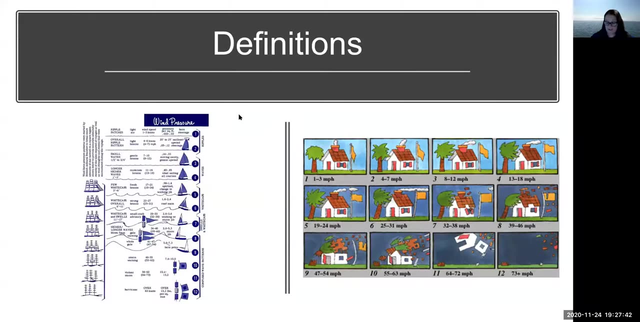 been slowly dropping throughout the day, studying at about a thousand and 5, which says that potentially there is a weather system on its way. So I can use a whole range of different sources online to take a look. So, as well as looking at what that weather is, I just need to have some indication of what those definitions mean, because the head 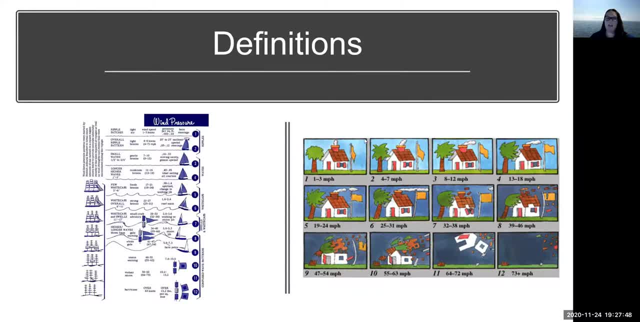 and the boots, and if you just jump closer here, if you just jump closer here, if you jump, you could. you could do the same Photos whenever with all different rejoice standings on. there are those five because on my inshore waters forecast it already started to give me some of those definitions. 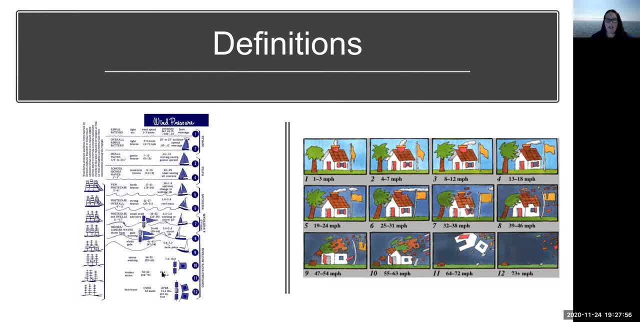 On my screen. here I've got a quick idea of what the brofit scale is. You can see the differences here between what sales I would have up, And you can also see on the right hand side here what sort of impact I would be expecting to see of different different wind strengths on my house and my flags. 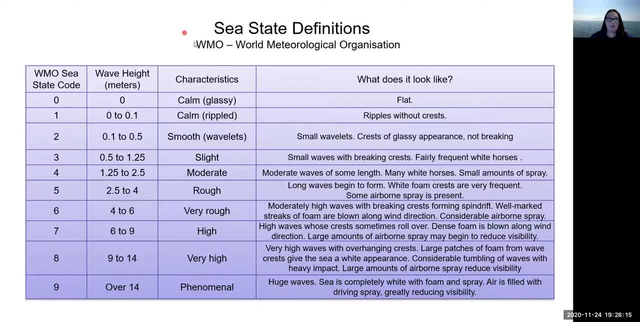 OK, if you were having a look there. So some really simple terminologies there And this is where we're looking at our sea state definitions. OK, we're really looking at up to sea state nine. So this is our World Meteorological Organization, And we're looking at wave heights everywhere, between zero all the way up to over 14 metres. 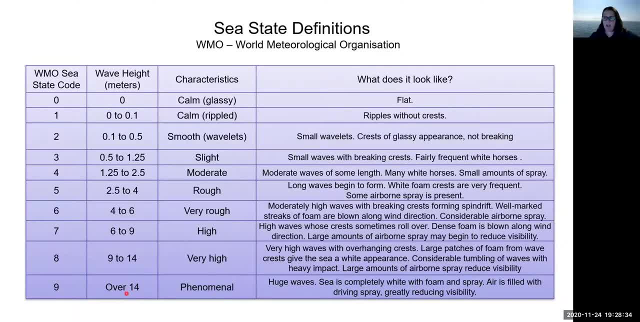 Once we're over 14 metres it's just phenomenal. OK, we kind of stop counting, All right, But then 14 metres is quite some wave. You know, that is a wave the size of a building, Let's face it. 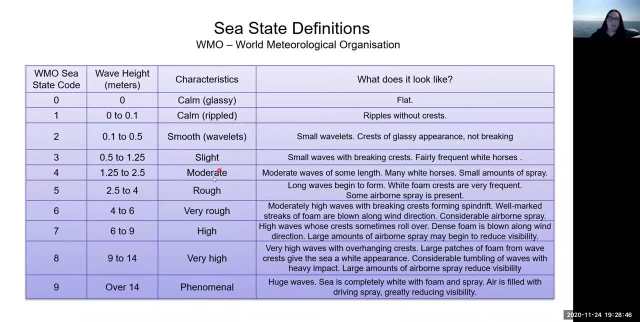 But what we're interested in is here. when we listen to people talk about moderate seas or rough seas, a rough sea is actually two and a half to four metres. That's pretty big. OK, quite a lot of people will probably sail in a moderate sea and say it was uncomfortable, for sure, but it probably wasn't quite verging on rough. 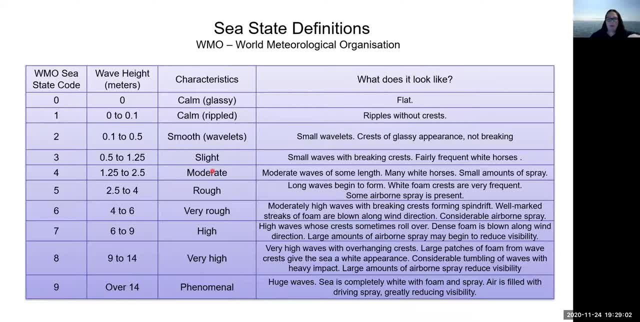 So some of these terms are going to be really simple. Do we need to remember exactly what all of the, the wave height of metres is? No, but I tend to remember that around sort of one to two metres I'm looking at a moderate sea, more than two metres. 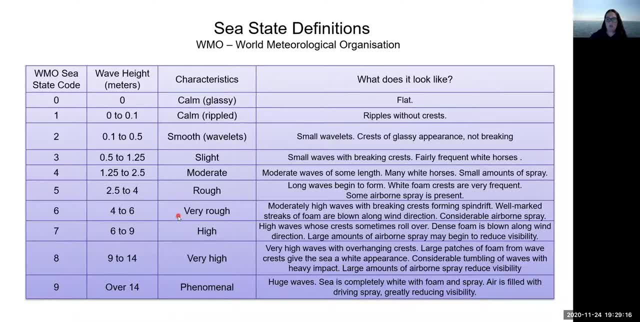 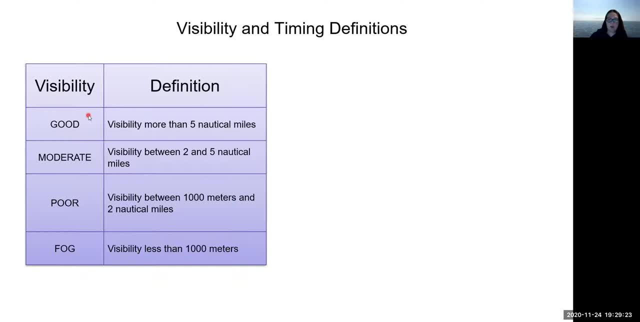 So two to three to four metres I'm looking at rough. Anything else is going to be pretty Uncomfortable. Also then my visibility, because that's one of the things that it shows up on my inshore waters. So what is good visibility looking at more than five nautical miles through moderate 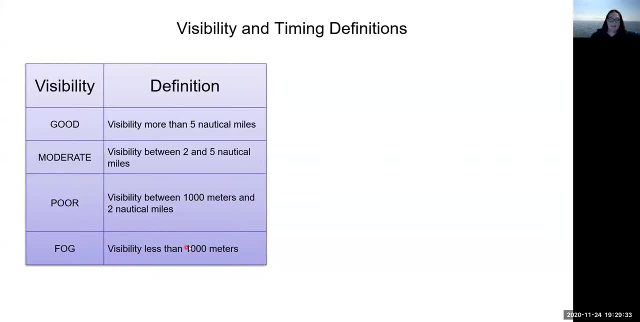 through poor and then all the way down to fog where we're looking at visibility of less than a thousand metres. So I can start to plan my trip. If it says moderate visibility, poor in places or poor in showers, I can start to understand realistically. what am I going to be expecting to be able to see? 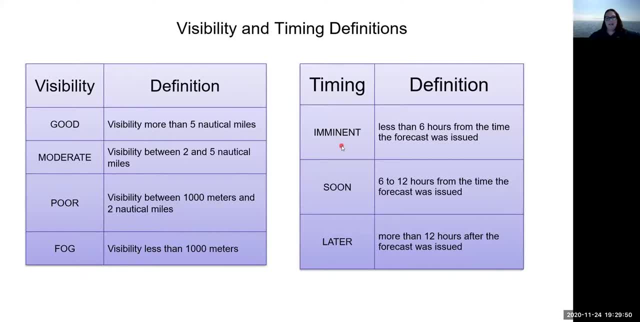 The timing is really important as well, particularly when we're listening to gale warnings, because if we're listening to anything that is imminent, so gale warning imminent. it is less than six hours from when that forecast was issued, not six hours from the time that you're listening to it or the time on your watch. 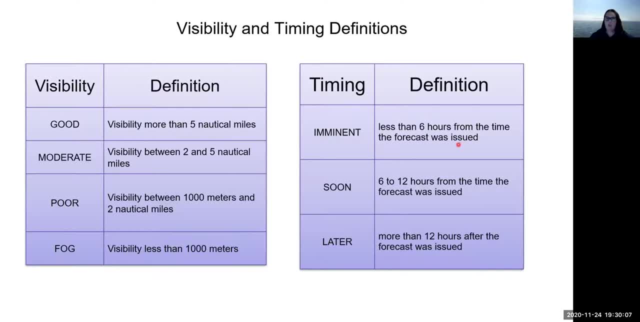 Six hours from when it was issued, And what I showed you earlier was that the inshore waters forecast list is done four times a day. So if it was issued at eighteen hundred, we're now at half past seven. So eighteen hundred. Anything imminent would be between eighteen hundred and midnight. 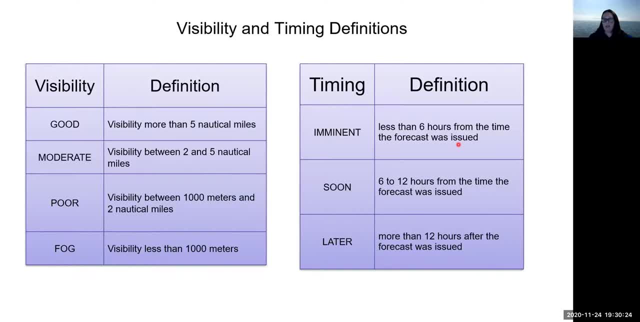 Anything soon, then we'd be looking at midnight onwards and anything later. we'd be looking at more than 12 hours then from when the forecast was issued. So it's really important that you understand that these timings are to do with when the forecast was issued. 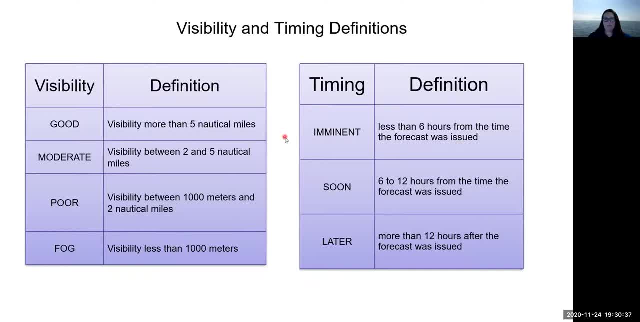 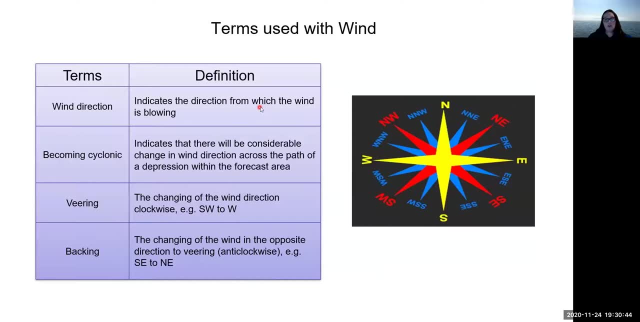 not when you might be hearing that particular forecast. When we're looking at terms for using our wind, then we're looking at our wind direction. is the direction that the wind comes from? OK, we know where the wind comes from. We're not so sure where the wind is going to take. 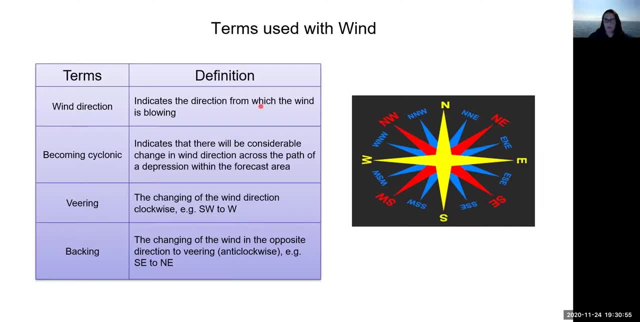 Lots of things can affect that land, all sorts of gradient winds. We can have divergence, convergence, all sorts of things. But we can be fairly certain that we know where the wind is coming from. So when we have southerly winds in the northern hemisphere, we're expecting them to be fairly warm. 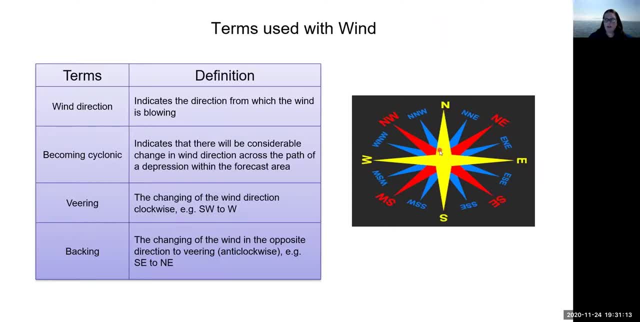 When we have northerly winds coming down from the Arctic, we're expecting them to be quite chilly. If we have weather that terms becoming cyclonic, then we're looking at a considerable change in the wind direction across the path of a depression. Sorry, within the whole forecast area. 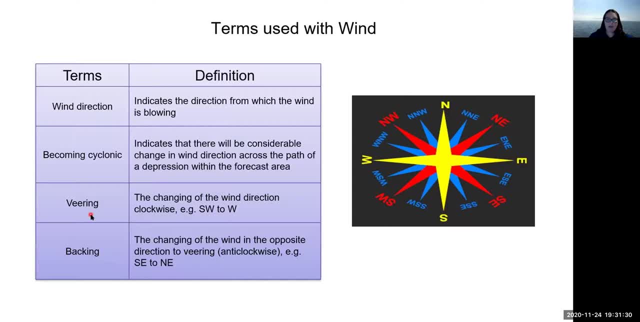 But also our veering wind. We'll talk about veering and backing when, when we talk about our pressure systems in the next session. we're looking at the change in the window action. So our viring wind is looking at going from perhaps the wind that's coming in south westerly to a wind that's coming in westerly. 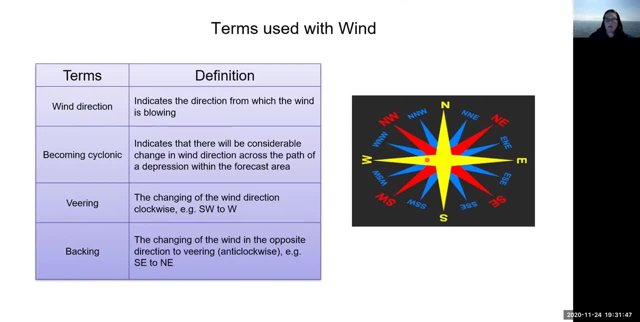 Or backing wind, then the opposite it, and I remember this one by thinking it's going back around the clock. okay, so the wind here is perhaps changing from a south easterly direction back around to a north easterly direction, and when we look at various different weather systems and weather fronts, we will start to see where the wind 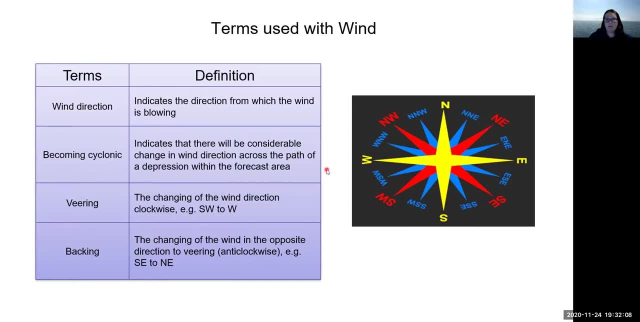 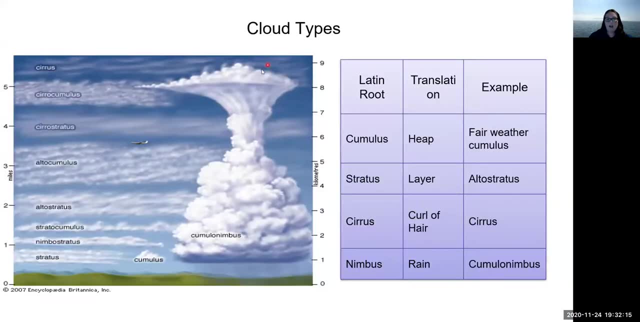 will veer and the wind will back as the weather front comes over us. So I did say we were going to have a quick look at some cloud types. okay, and our cloud types. really, although there's heaps and heaps of cloud types, there's only a certain number of genesis of cloud. okay, and we use the latin root. 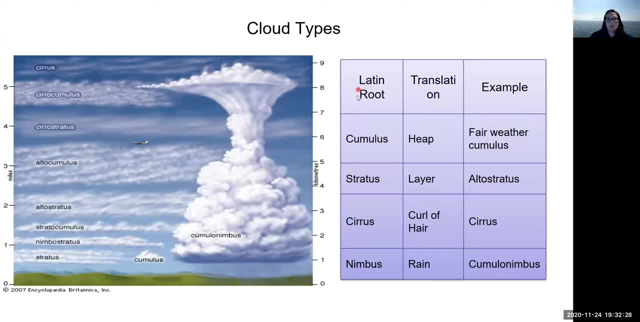 of the words to understand what that actually means. So if we have a cumulus cloud, we're talking about it being a heap. okay, so we've got a little cumulus cloud down here. I always think this is a bit like, you see, when, when the simpsons comes on, you see the little clouds pop up at the front of 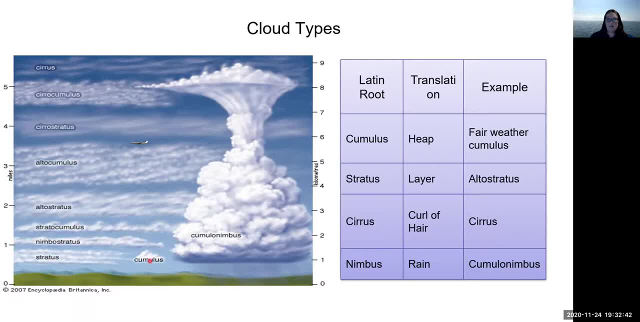 the simpsons, it's those lovely, fair, with a cumulus cloud Like we have here. okay, so a heap, as in a whole load, of what looks like a big chunk of cotton wool. then we have our stratus, which is our layer, okay, and we can have an example of alto stratus. so here, 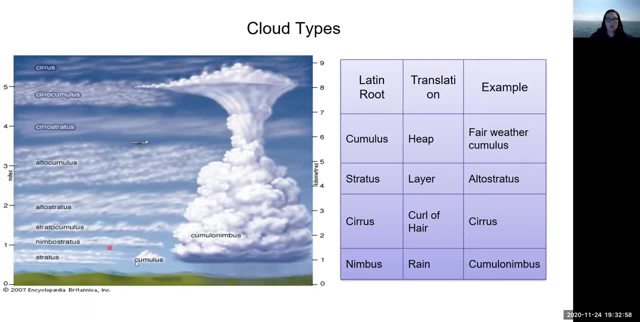 we've got mid-level layers, okay. so as soon as we start turning our clouds into a layer, we're going to add strato to them. so here we have a single cumulus cloud, yet here we have strato cumulus, a layer of cumulus cloud, a layer of heaped clouds. 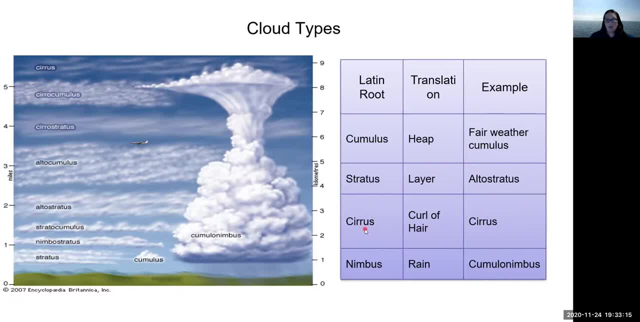 Then, further up, we go up to the top. here we're looking at cirrus, where we're looking at it being a curl of hair. these are these high level clouds which are really the ice crystals- okay, very pretty patterns, but they're lovely little ice crystals that we'll see at the top, and then the ones that 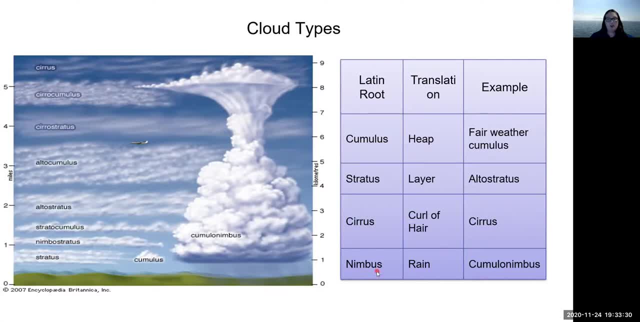 we probably don't like so much the nimbus clouds. okay, so these are our rain bearing clouds, so anything that's got nimbus or nimbo will be rain bearing. so here we've got a very large cumulus nimbus cloud. so it is a heap. 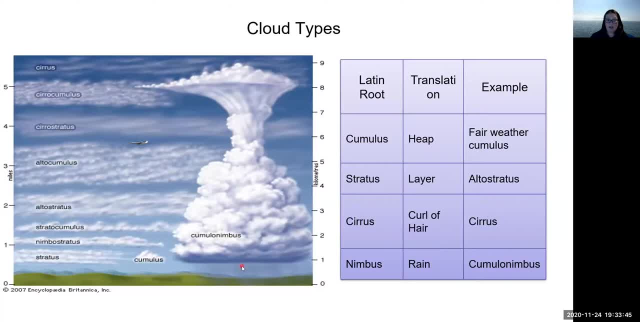 Cumulus and nimbus. it's rain bearing. you can see the rain coming out of the bottom of it. there we've also got a nimbus stratus on the left hand side, so we've got a layer of rain bearing cloud and if you can remember the four of these, then you can pretty much put all of the different clouds together. 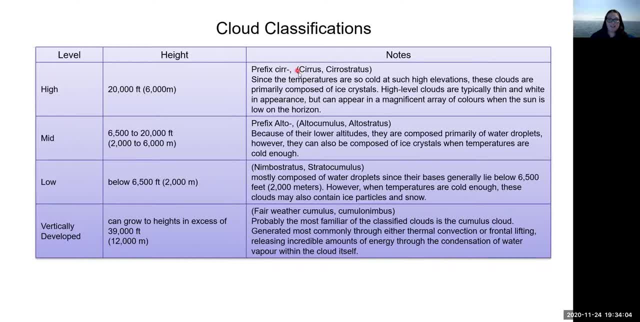 So how high are we looking? well, when we look at our cirrus, then so cirrus cirrustratus, we're up at around 6,000 meters, 20,000 feet. these are the ice crystals that we're looking at. okay, primarily composed of ice crystals, because of how high they. 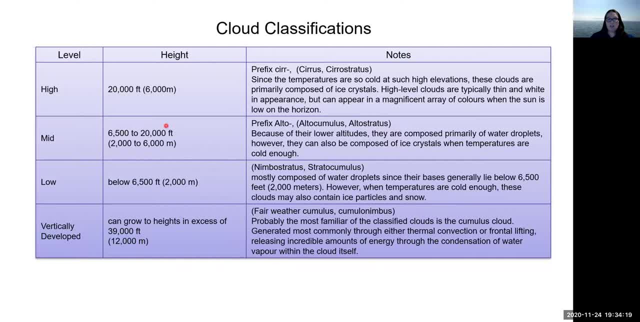 are in the atmosphere, Our mid-level clouds. they're between 2 and 6,000 meters and we're looking at alto, so that's our mid, so alto, coming from sort of the mid-level voice, if you like. and we've also got our lower clouds then down below 2,000 meters, mostly composed of water droplets. then, because of 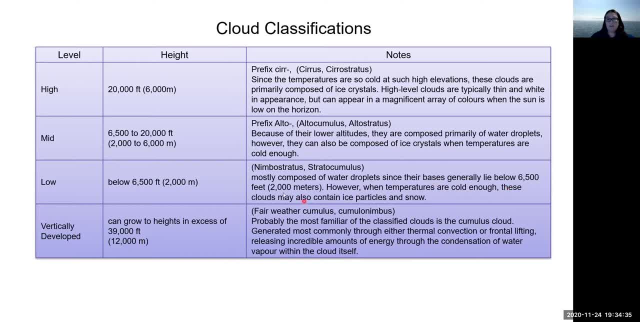 how low they are, and when the temperature gets cold enough, then these can also contain ice particles and snow. okay, and our vertically developed clouds are those clouds that are very, very tall ones, where we would look at a huge lot of thermal convection, frontal lifting with lots and lots of energy, and generally we're looking at vertically developed clouds turning. 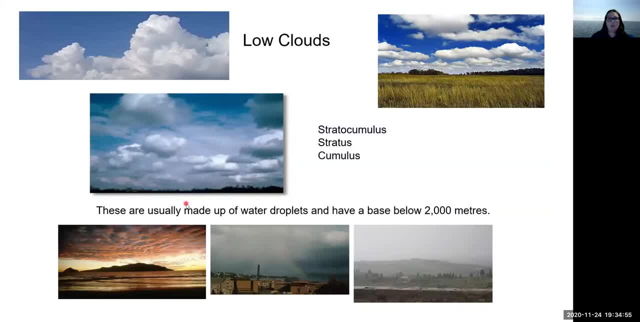 into storm systems, so certainly thunderstorms. So some pictures for you to give you an idea of what they actually look like. we've got low level clouds then, where we've got cumulus, strata, strata, cumulus, these ones. here we've got some individual cumulus clouds turning into a bit of a layer there. 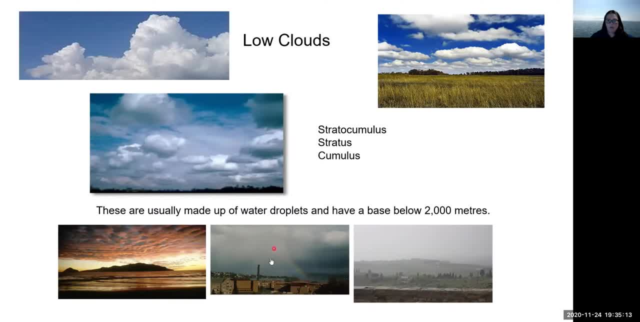 we can see our layer down here and we've got a little bit of a layer down here and we've got a layer down in the bottom left hand corner. we've got some rain in this one so we can have a rain bearing cloud, and we've got our lower level ones made up of water droplets, usually below about 2,000. 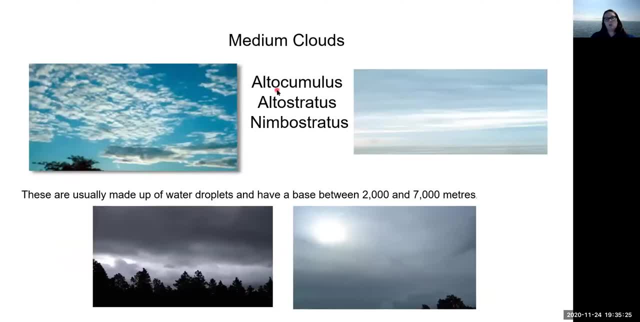 meters on medium clouds. then we said about our alto clouds: again, think that alto voice, alto cumulus, alto stratus and limbo stratus. whether we're looking at something like this, this is looking fairly rain bearing in there with all that darkness, okay, and we can have alto cumulus where.